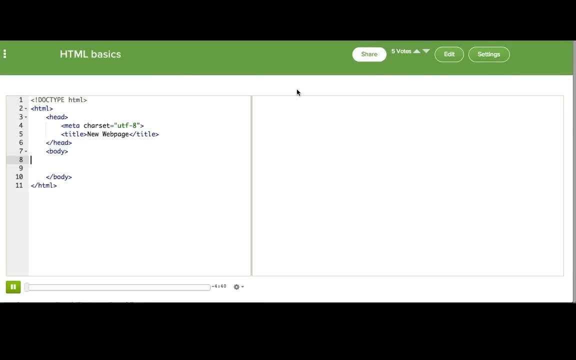 Welcome to my web page. I know it's not a very exciting web page. It's completely blank, But every web page starts that way, and I'll show you how to build up this page soon. First, though, give me a minute to show you around the skeleton of a blank web page. 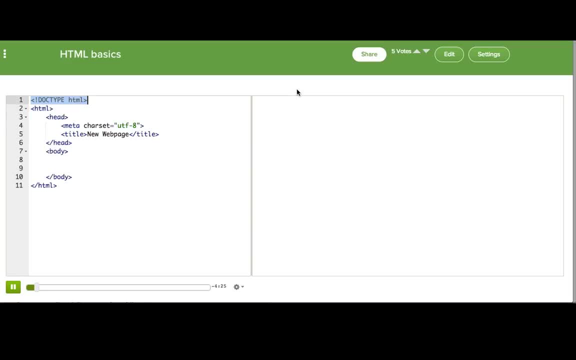 Every web page starts with this funny looking thing called a doctype at the top, And this is just a signal to the browser that this web page is written in modern HTML and not a kludgy old, weird HTML Next to the very first tag of the page. 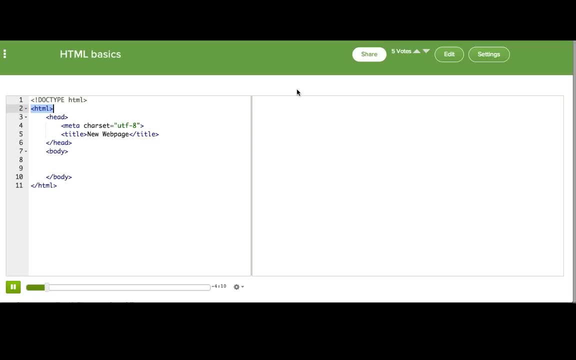 HTML is a markup language, so it's all about tags, And a tag is one of these things that starts with an angle bracket and ends with another angle bracket, Or, if you like math, you might think of them as less than and greater than signs. 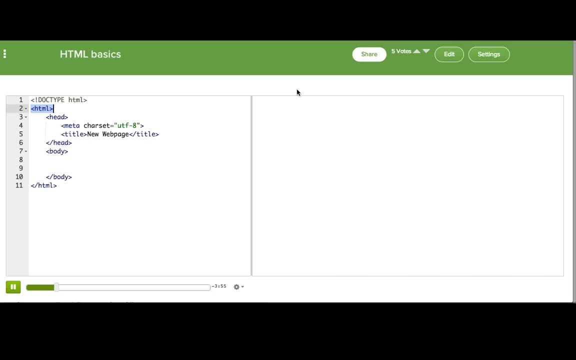 The first tag of every page is always that HTML tag right under the doctype. This one is the start HTML tag, and then at the bottom there's this end HTML tag, Which is the same, except for this backslash, which is really important. 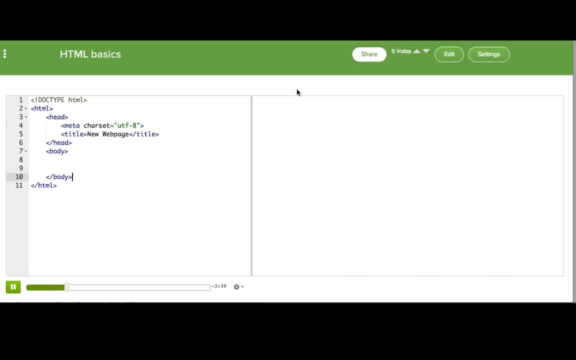 The HTML tag needs to contain every other tag that makes up this web page, And that's why we don't have the end HTML tag until the bottom. A lot of HTML tags come in pairs like this, but not all of them. Okay, Underneath HTML, there's always a head tag. 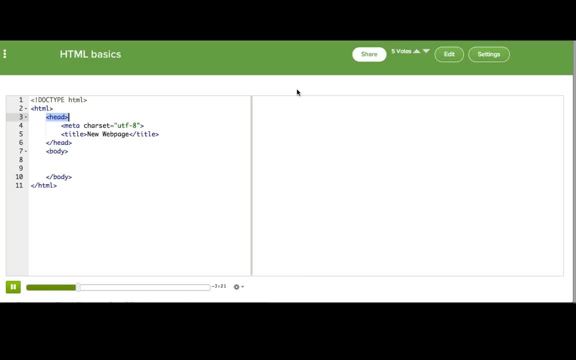 And that contains tags that helps the browser render the page but doesn't contain anything the user actually sees. There's this meta tag. There's this meta tag That gives the browser more details about how to render the page, For example, if you're using common characters, like from English language. 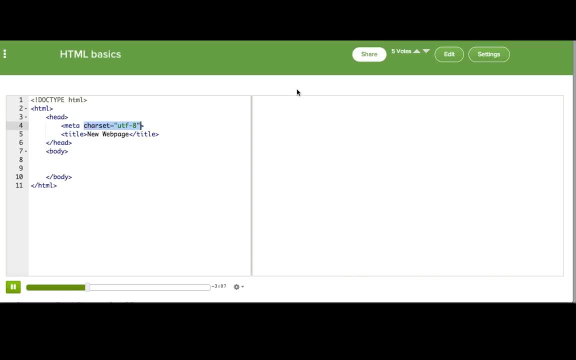 and not harder to render characters like from the Arabic language, then you should have meta char set equals UTF-8.. Then there's this title tag which the browser uses to decide the title of the page And this is what shows in the tab on top of browsers and in bookmarks and in search results. 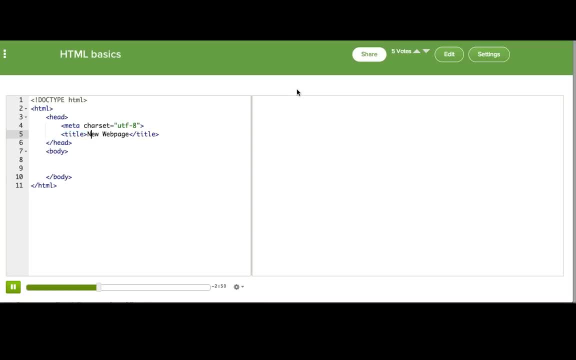 And here on Khan Academy, the title shows up above our web page. Let me change the title. I'm going to make a page all about rabbits, So I'll say all about rabbits And maybe you can actually see as it changes above. 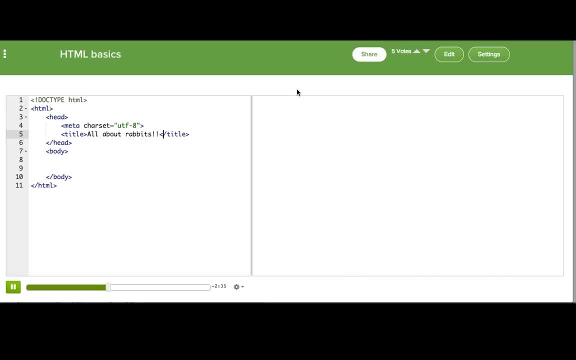 Nice. Okay, Now we're done with these details. So we end the head tag and move on to the tag where it's all going to happen: the body tag. It's pretty boring right now. just the start and the end. Okay, What should I add? 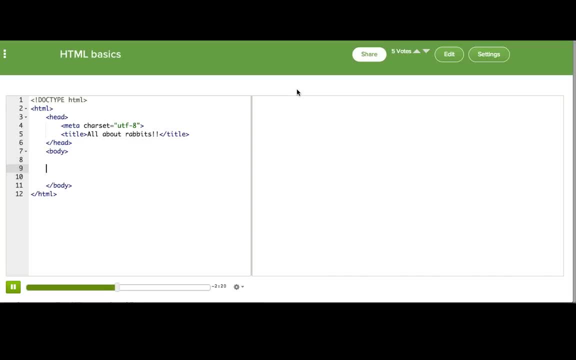 Well, I'm making a web page about rabbits, so I should probably declare that in a big old headline at the top. To add a headline, we use the H1 tag And all about rabbits. Great. Actually, we have six tags that we can use for headlines. 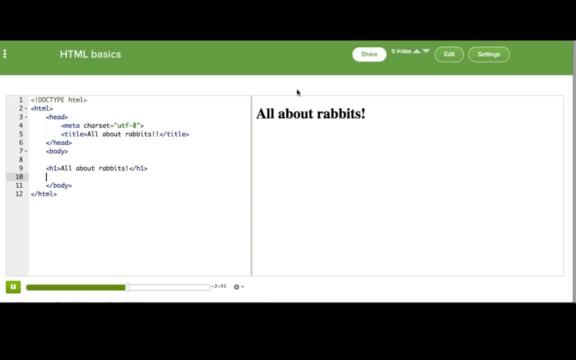 H1, H2, H3, H4, H5, and H6.. The H1 is for the most important headlines on the page and H6 is the least important. Let me add a few more headlines for other sections. 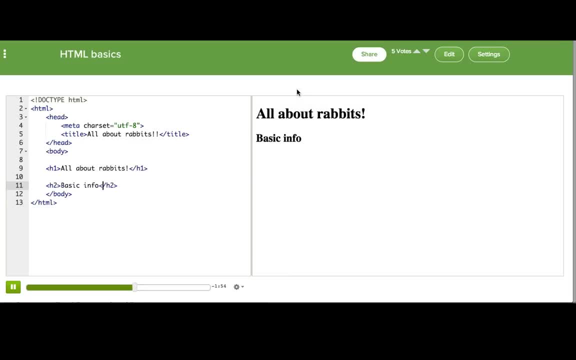 and I'll use an H2, since these are slightly less important sections And some songs: Okay, Great, Now let's add some information. Well, my target audience for this page is aliens that have never seen rabbits, so I better give them a good description of rabbits. 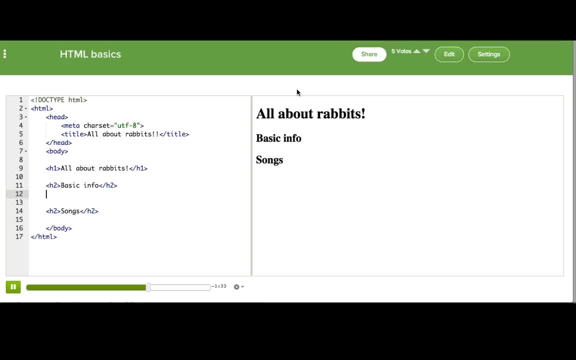 In fact, I think I need a whole paragraph of information. How can I mark up a paragraph in HTML With the P tag, of course? So we put in that P tag and then I'm just going to go ahead and paste in the information. 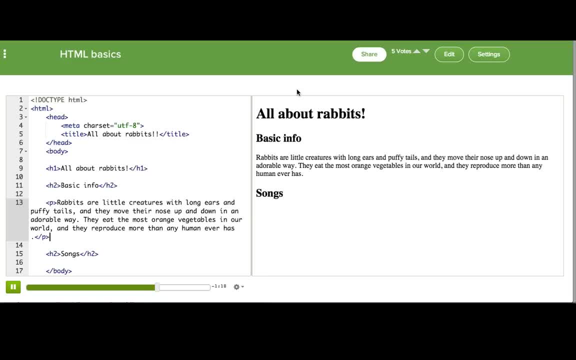 so that you don't have to watch me type the whole thing. Beautiful, All right. now the aliens will need a song to greet the rabbits with, so I'll give them lyrics to my personal favorite and once again use that P tag for it. 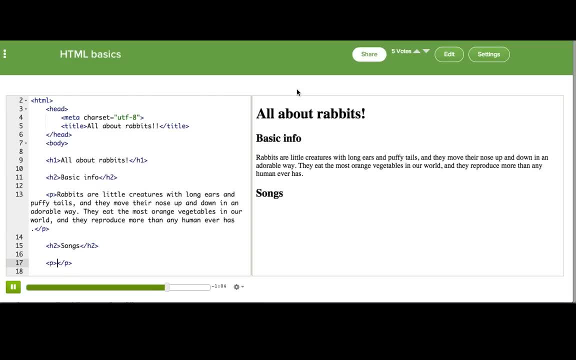 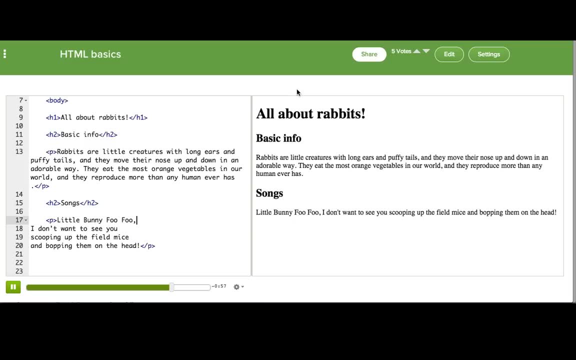 and paste in the song Little bunny foo foo. Ah, such a good song, But uh-oh, it's showing up all on the same line. How will the aliens know when to pause? Why didn't the browser render the line breaks that I put in here? 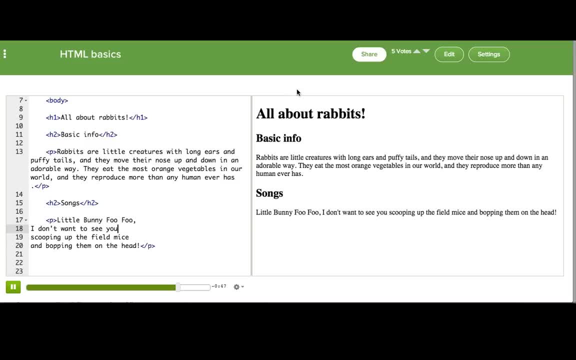 Well, actually, browsers mostly ignore line breaks in whitespace in your HTML and if we want the browser to render a line break, we have to tell it explicitly using another tag. The BR tag stands for break. So we'll go through and add BRs after each line.